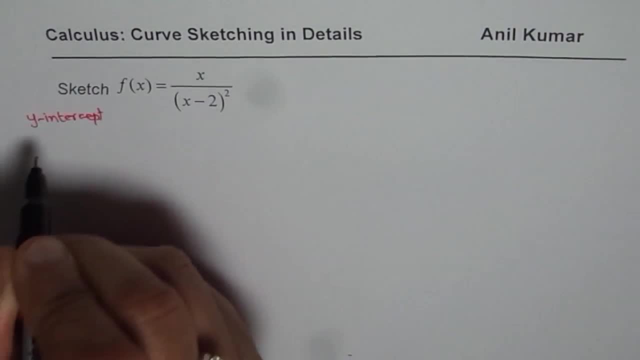 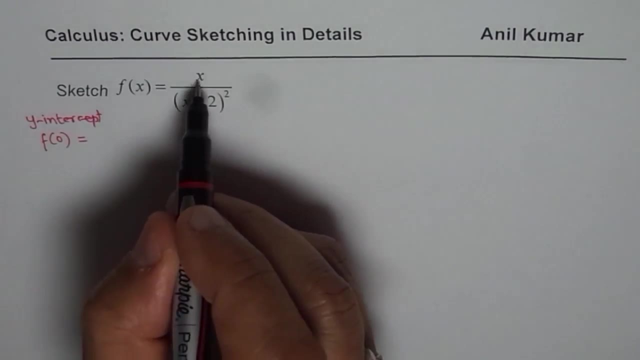 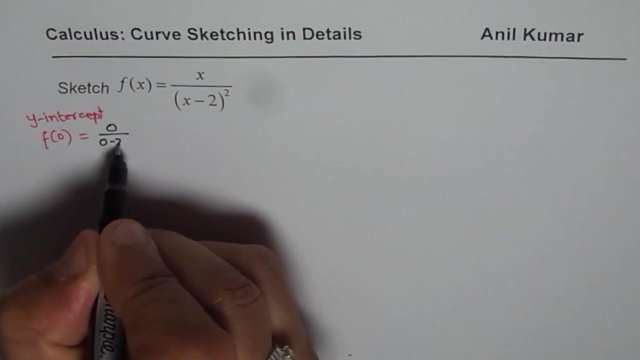 Y intercept is a point where x is equals to 0. That means we need to find the value where x is 0. That means f of 0. If I substitute 0 here, then what do I get? I get 0 over 0 minus 2. 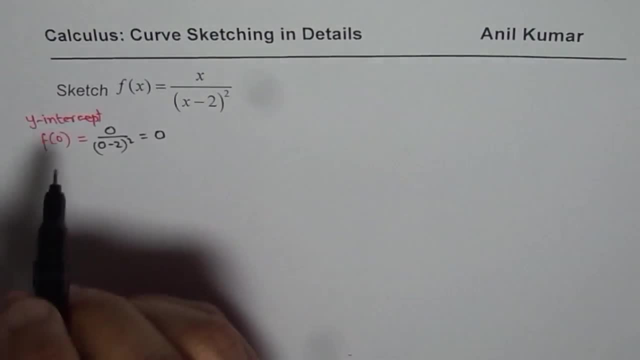 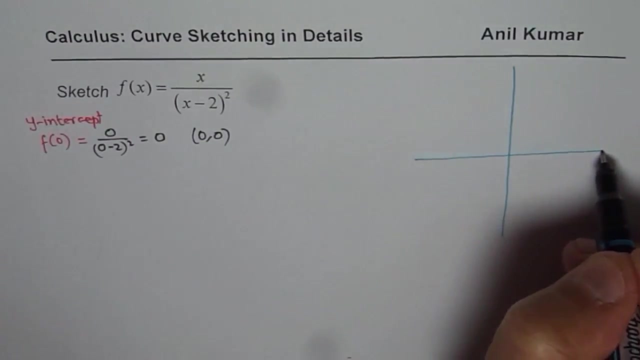 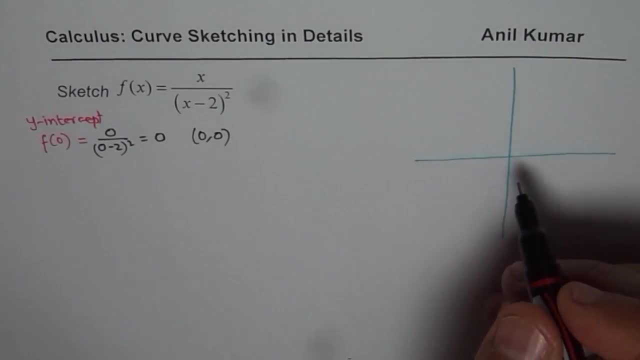 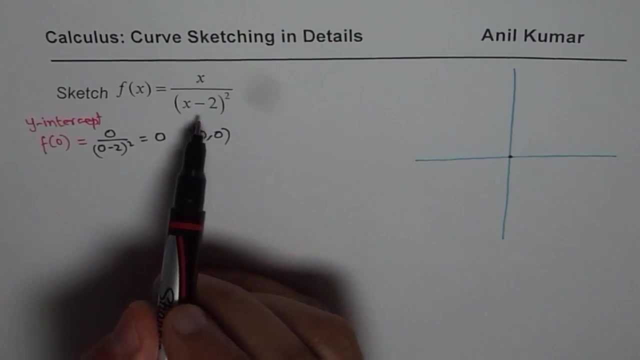 Simultaneously. That will help us to see how the picture is developing. right? So we got the first point, which is also the y intercept and x intercept, and that is at origin, right? So this is our first point. Now, when you observe this equation, you see that there is a vertical 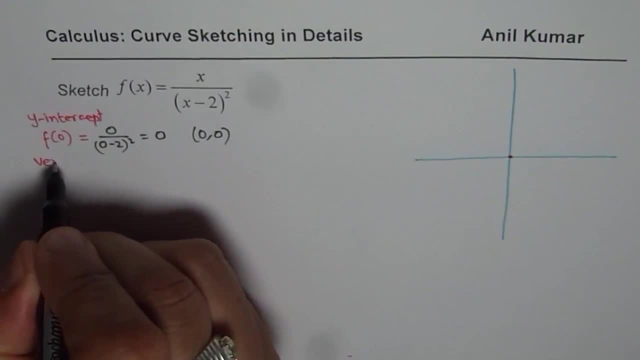 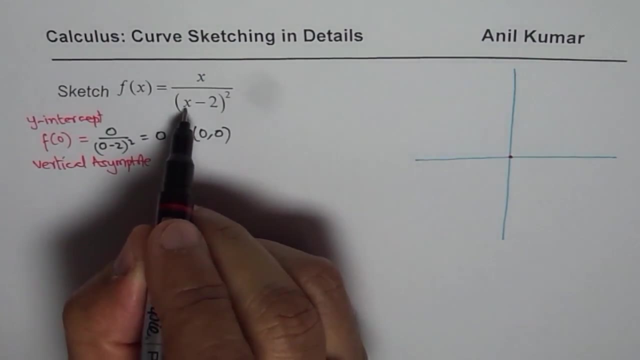 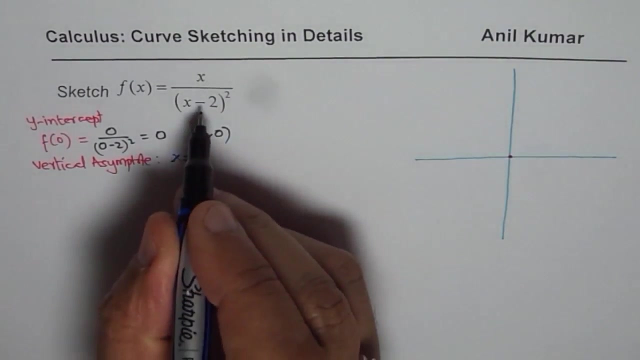 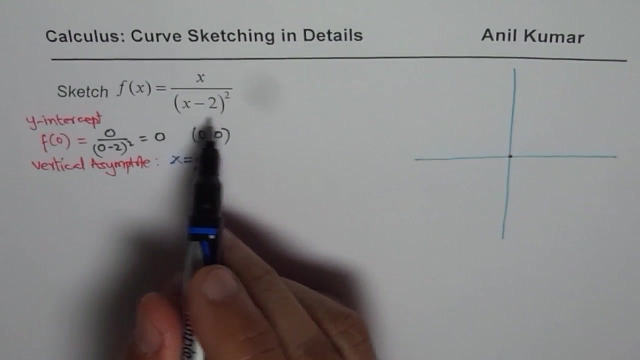 asymptote. right, So we can go for vertical asymptote. Vertical asymptote is at x equals to 2, right, So vertical asymptote is at x equals to 2.. Since at x equals to 2, denominator is 0, right, So I mean x equals to 2.. Denominator is 0.. So how do we find it? 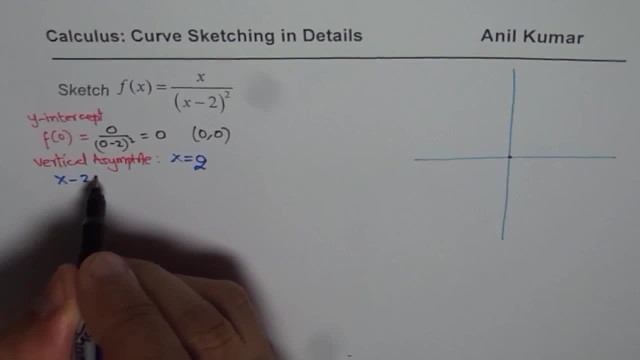 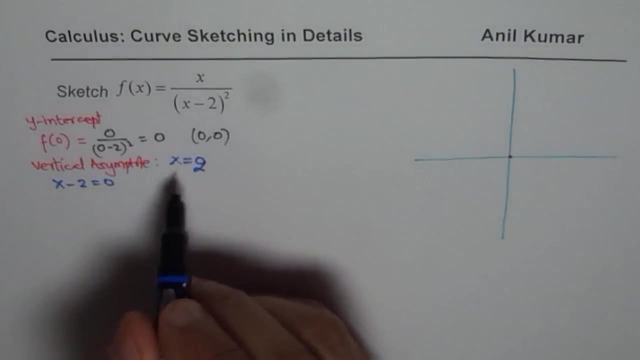 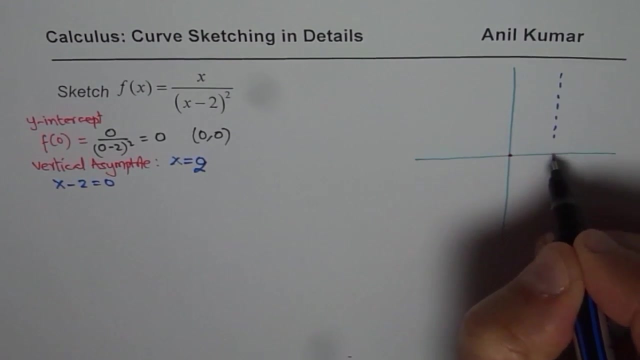 Equate the denominator to 0 and solve for it. So we do: x minus 2 equals to 0, and that gives us x equals to 2.. So what we can do now here is, we can plot the vertical asymptote Also, which is at 2.. So let me sketch a dotted line, vertical dotted line here. So that is. 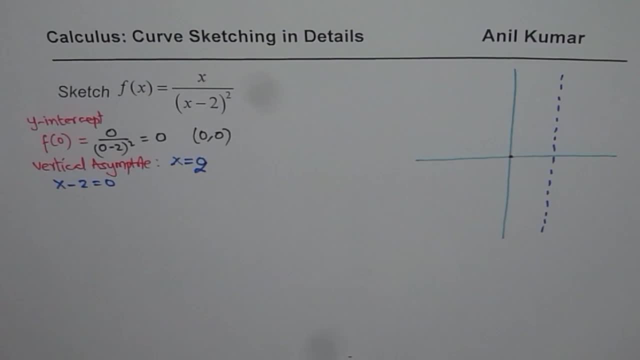 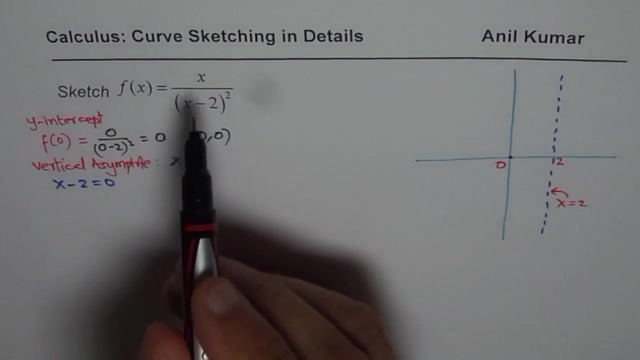 let us say x equals to 2, right, So we get this vertical asymptote and we'll say that this is x equals to 2, the vertical asymptote. right, So that point is 2.. This is origin for us. okay, Now let us look into the horizontal asymptote. 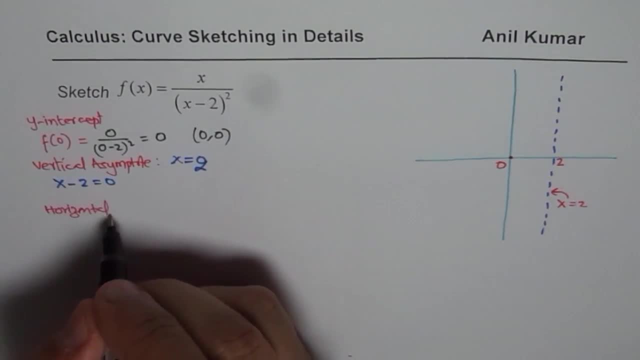 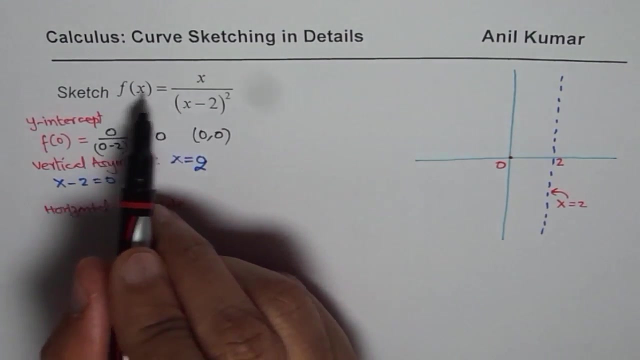 Since the degree of denominator is higher than the numerator, what do you expect? You expect that as x becomes increasingly large, as x approaches infinity, positive or negative, the function approaches 0, correct. So function approaches 0 and therefore we do have a. 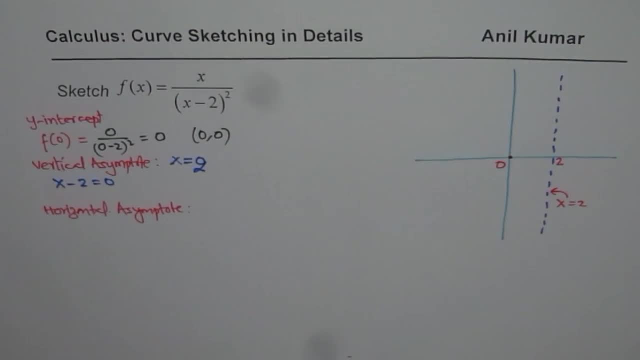 horizontal asymptote. and this horizontal asymptote will be: y equals to 0, right. So the function approaches 0 as x approaches positive or negative infinity. So let me sketch this also here, showing this dotted line along the x-axis as our horizontal. 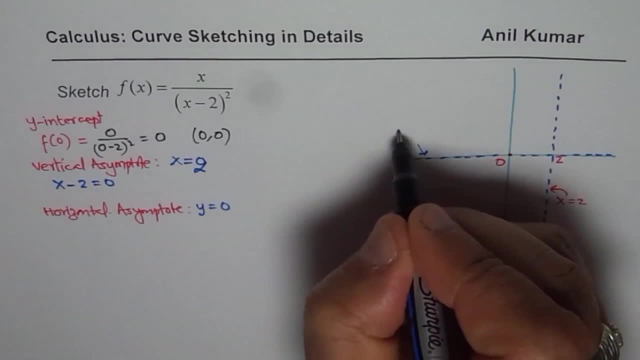 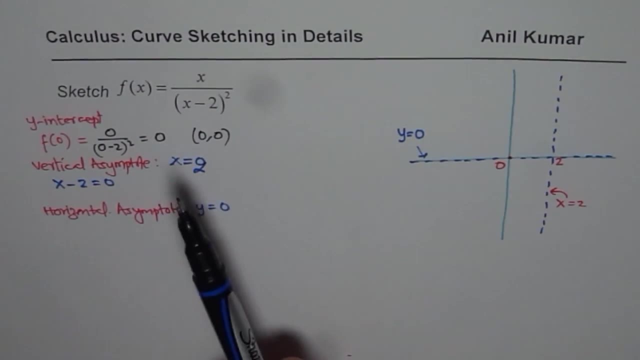 asymptote correct. So this becomes horizontal asymptote y equals to 0.. Now, once you find horizontal and vertical asymptotes, it is important to see behavior near the asymptote right. So let us now check For both vertical asymptote and horizontal asymptote. In vertical asymptote we'll approach. 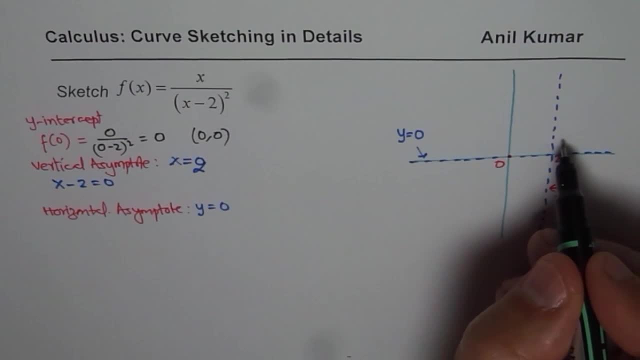 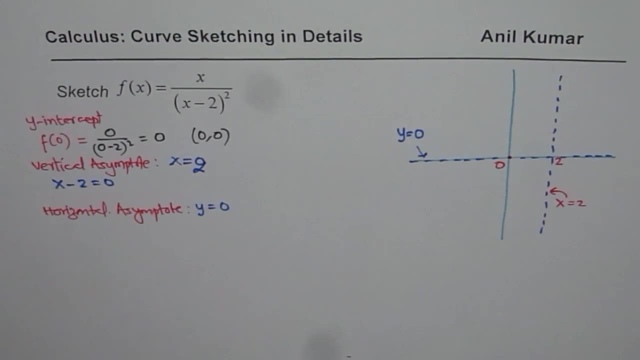 2 from left and right side and see whether we approach negative infinity or positive infinity, right? So let's check the behavior. now Let me use a different in to write behavior near asymptote, right? So we'll say behavior near asymptote. 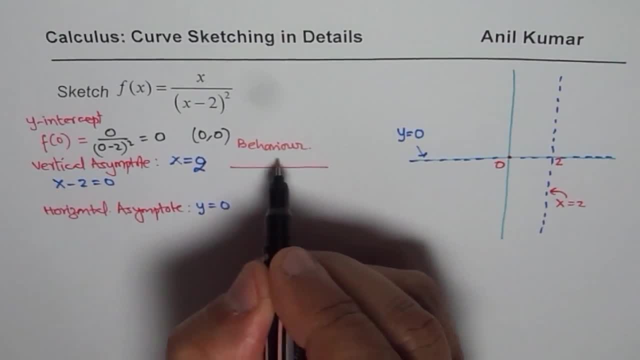 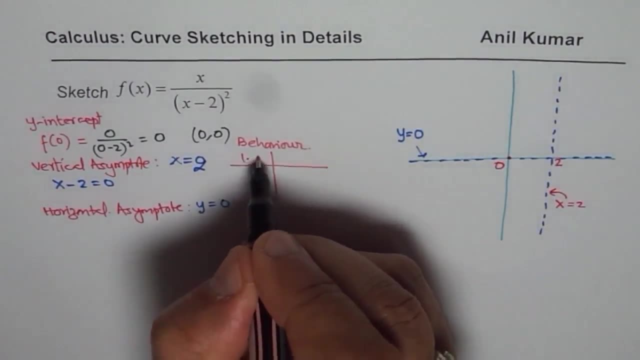 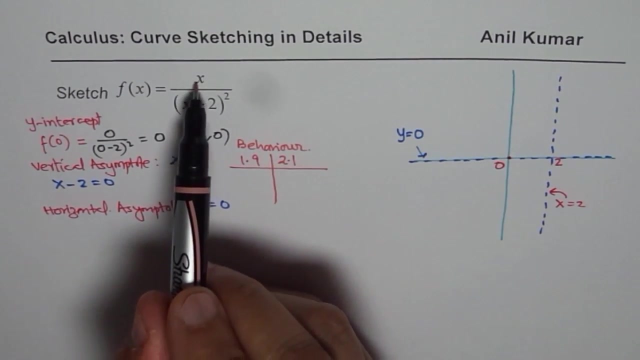 So to check the behavior, we'll consider two points, one on the left side and one on the right side. So left side point could be 1.9, right side point could be 2.1. Now if I substitute 1.9 here, it is positive. denominator is also positive, so that approaches positive. 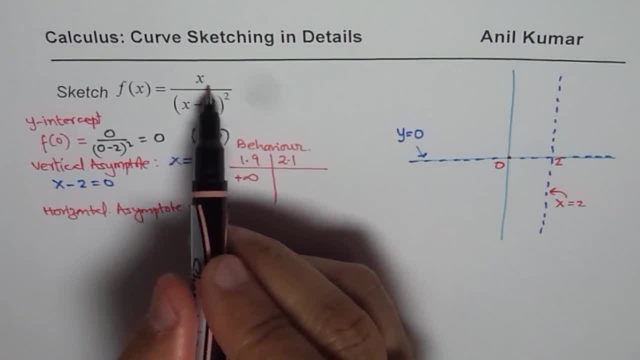 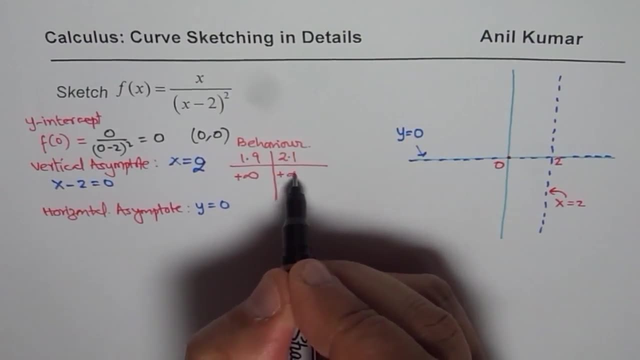 infinity. If I substitute 2.1 here and here, in that case it is positive. So here again I substitute, it will approach again positive infinity, right? So that is the behavior. What we notice is that the graph of the function 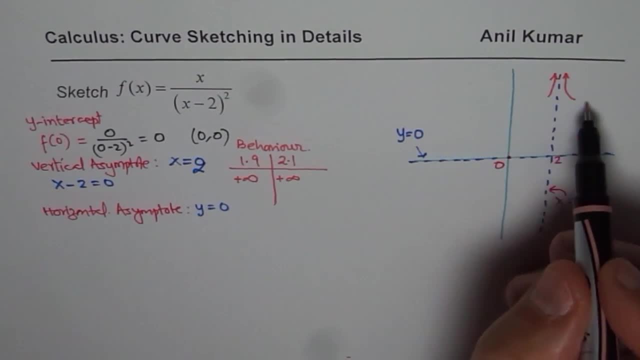 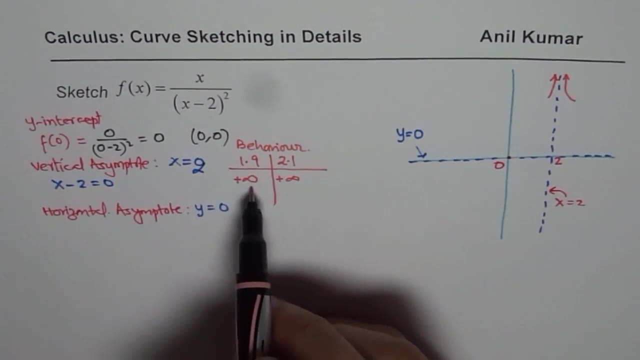 moves towards positive infinity when we approach 2 from either side. So you can actually substitute this value here in the calculator and check, So you'll get positively large value right. We'll do the same calculation for the horizontal asymptote also and try to figure out. 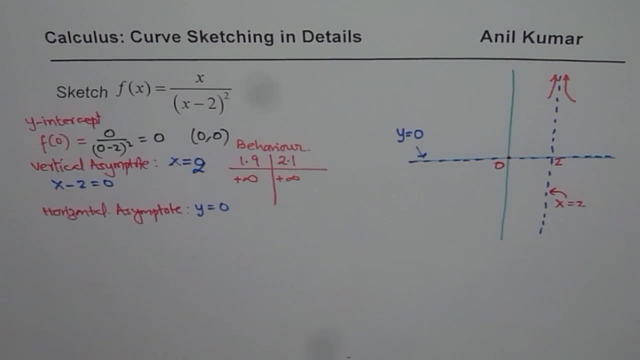 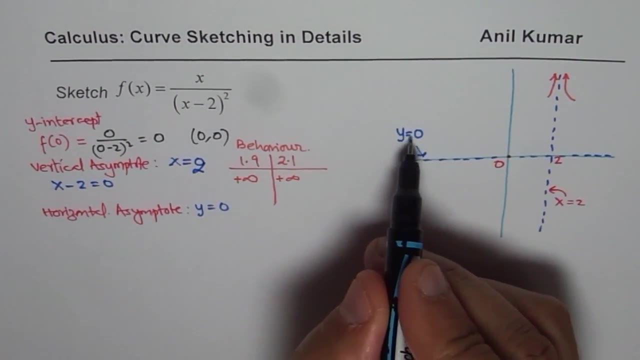 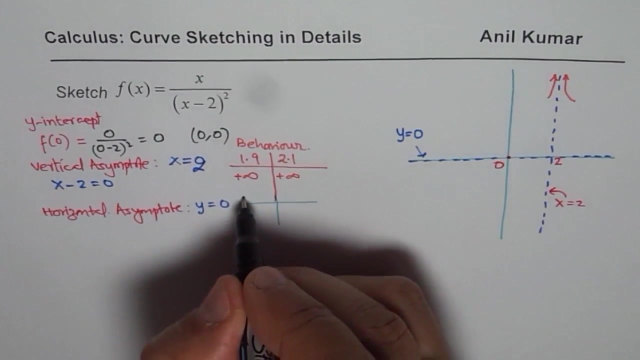 how will the function approach the horizontal asymptote, whether it goes from above or below right. So in that case, we know horizontal asymptote is 0.. So if I substitute a value, let me substitute. let us say minus 100 and plus 100. 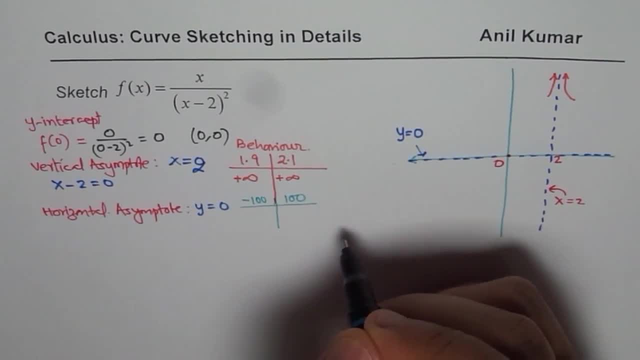 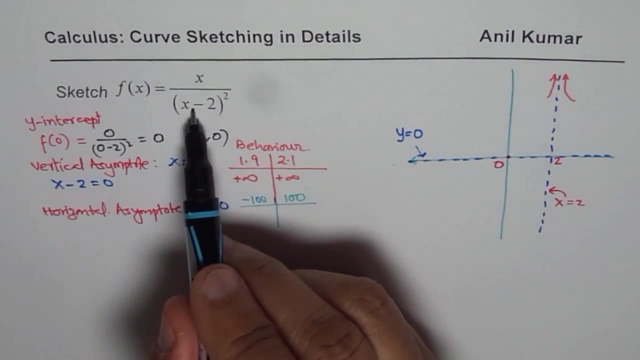 So minus 100 for us is kind of negative. infinity right, Very large value As compared to 2, minus 100 is extremely large. Denominator you see is positive, But with negative 100, numerator will become negative. 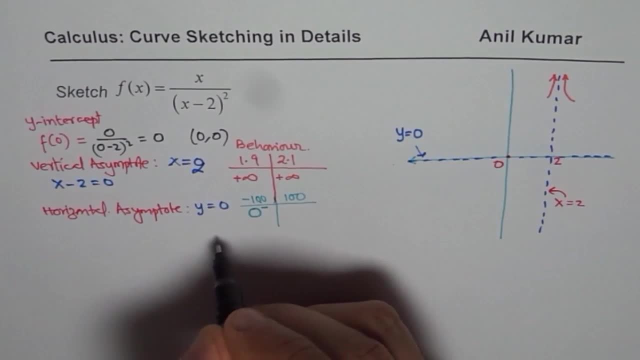 So we will approach 0, but from the negative side. So I'm trying to say that this is going to approach like this. Do you see that? From the negative side. But if I substitute 100 in my equation, I'll get again 0,. 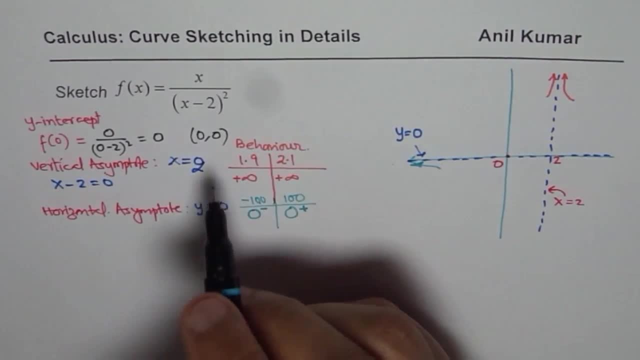 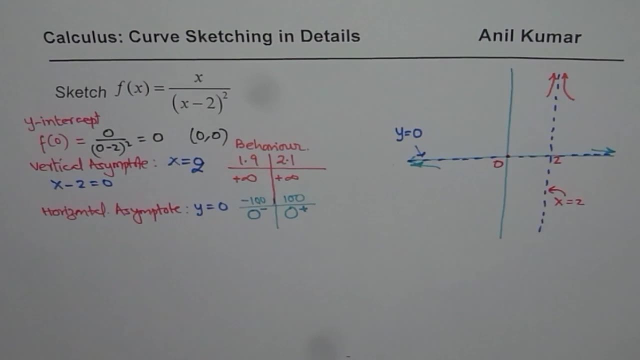 but it'll be from the positive side, Since the numerator is positive, denominator is always positive, So the end behavior is kind of like this. So what we have here that we do have x and y intercepts. So the graph could come like this: 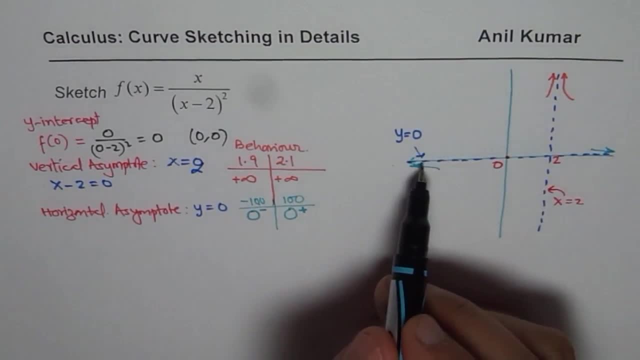 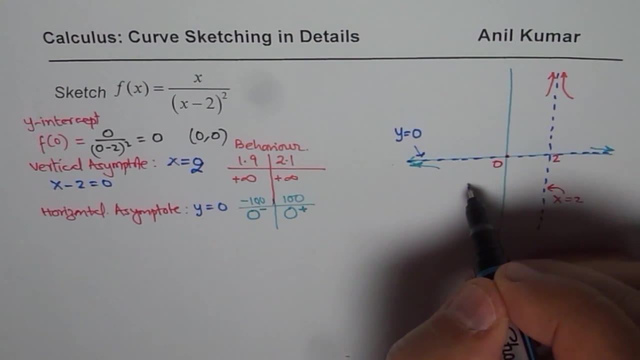 Now, since it is going to approach horizontal asymptote, which is y equals to 0 for negative infinity, it has to turn somewhere and that turning will lead to a minimum value And also it will lead to change in concavity. So let us now analyze the first and the second derivative right. 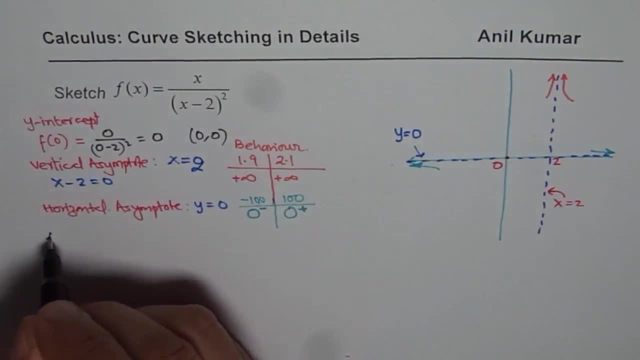 So function is given to us. Let us find the first derivative of the function. f prime x will be. we'll apply the quotient rule, square of the denominator, which is x minus 2, to the power of 4, derivative of x is 1,. 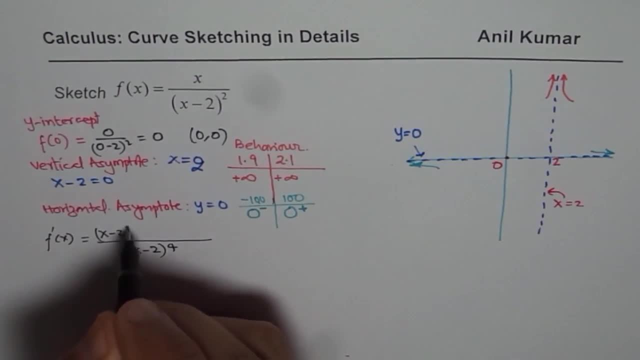 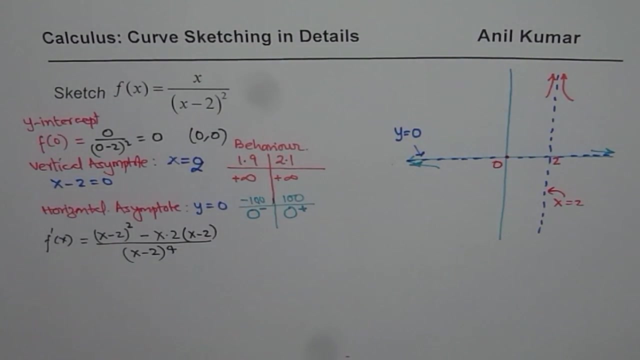 times x minus 2 whole square. So we get x minus 2 whole square minus x times derivative of this function, which is times 2 times x minus 2, right, So x minus 2.. So that is what you get in the numerator. 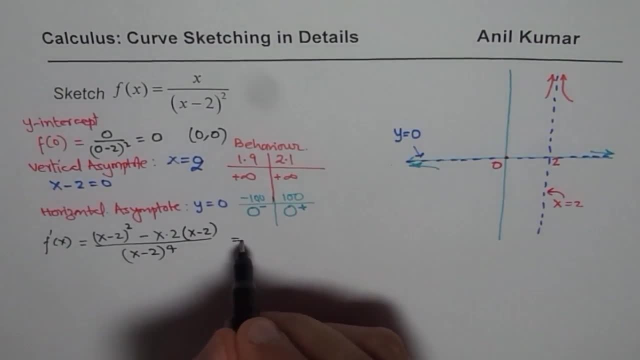 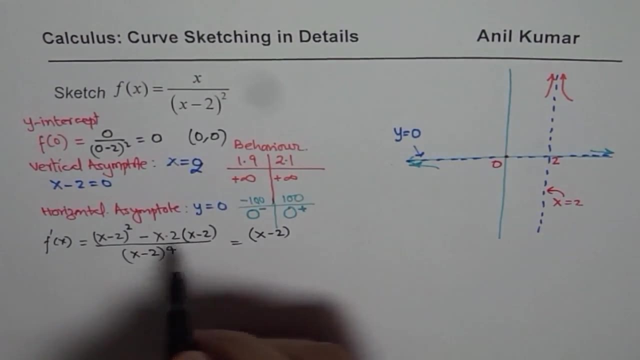 Now we can actually simplify this a bit, Taking x minus 2 common in the numerator. let's say x minus 2 is common in the numerator. What we get here is x minus 2 from the first term and 2 x. 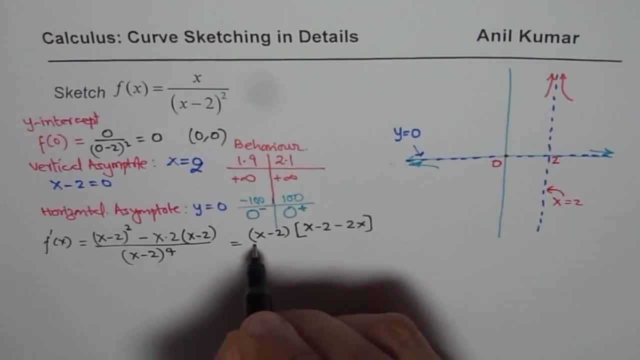 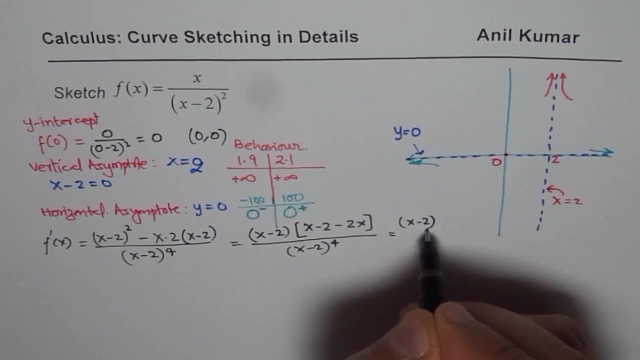 minus 2, x, rather from the second term, divided by. And here Here we get x minus 2. times x minus 2x is minus x. So we get minus x minus 2, right, So that is what you get in the numerator divided by x minus 2 to the power of 4.. 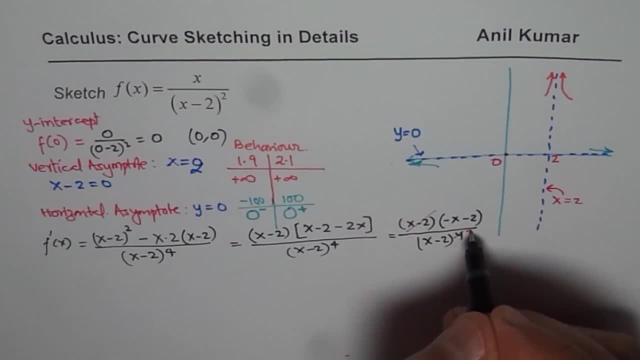 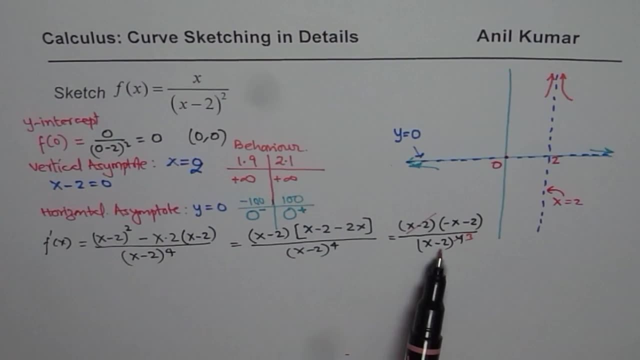 So this could be further reduced. We could actually change this to q, correct? So we get minus x minus 2 over x minus 2.. So that gives us two critical points, right? We will analyze these two critical points. 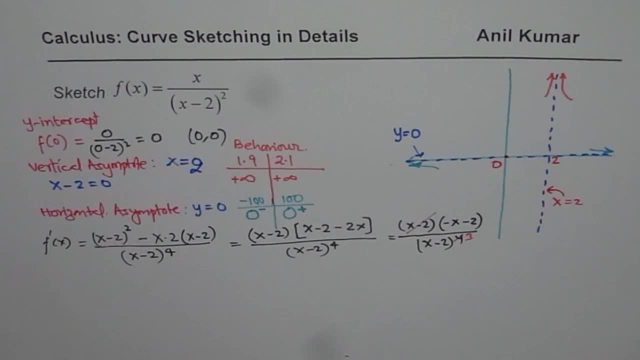 So the critical points for us are at: x equals to plus 2 and x equals to minus 2, right? So plus 2 from here and minus 2 from there. So these are the two critical points for us, correct? 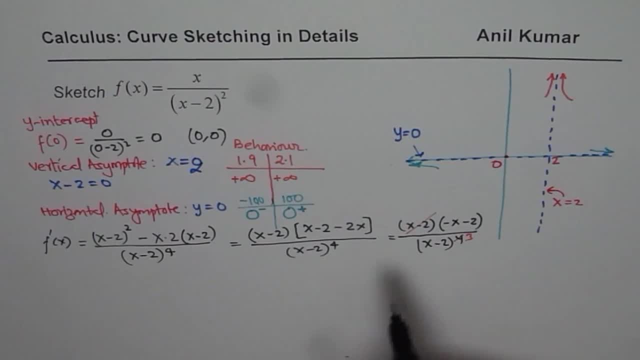 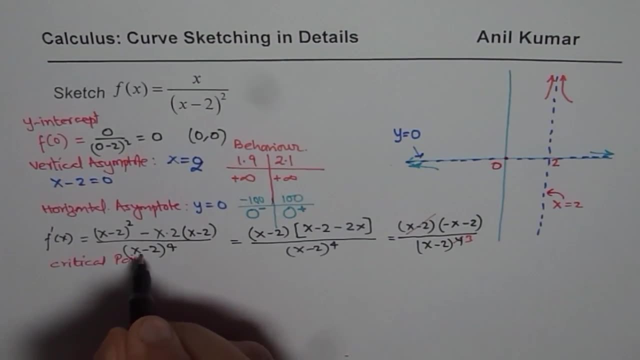 So we can write from here that the critical points are x plus 2 over x minus 2 to the power of 4.. So that gives us two critical points, right? So critical points to analyze are: at x equals to plus minus 2, right. 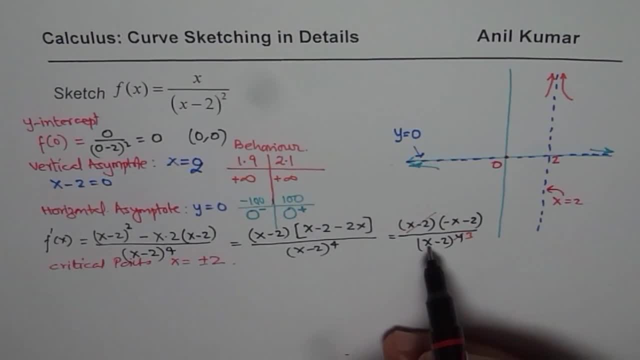 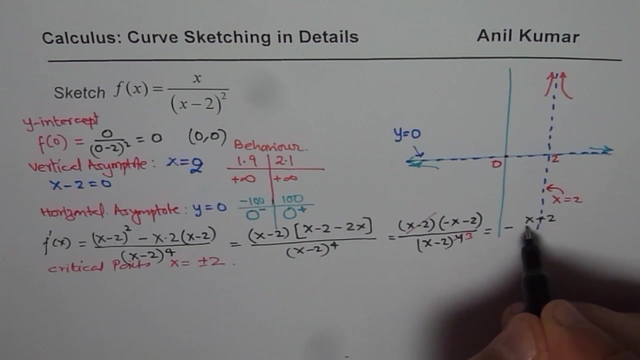 So these are the critical points. Plus 2 will give us undefined derivative and minus 2 will give us 0, right. So these are the two critical points. Let me rewrite this expression as minus of x plus 2 divided by x minus 2.. 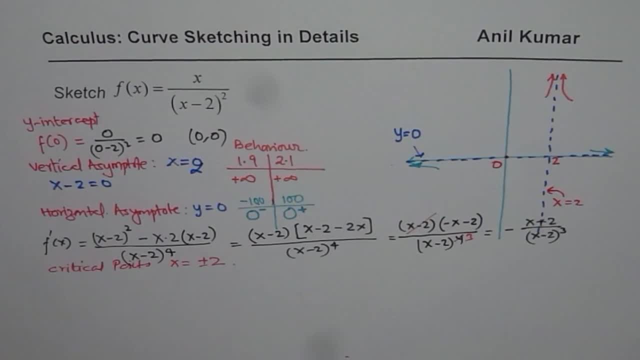 Holes q correct. So that is the first derivative and these are the two critical points for us. Now let us analyze these critical points. So analyzing critical points for the first derivative will help us find the maximum or local maximum. 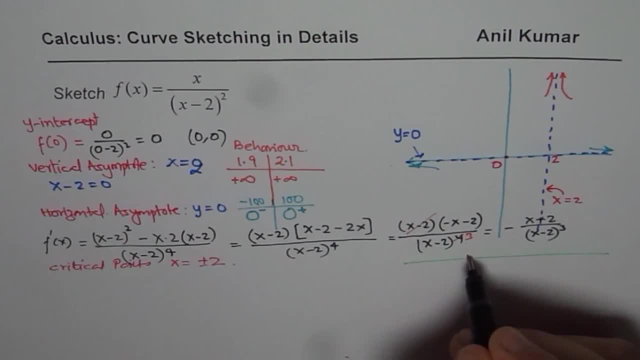 So what we have here is one at minus 2, right, The other one is at plus 2. So we can take a test point on either side of these. So if we take a test point on either side of these critical points, it could be minus 3,, 0 and 3.. 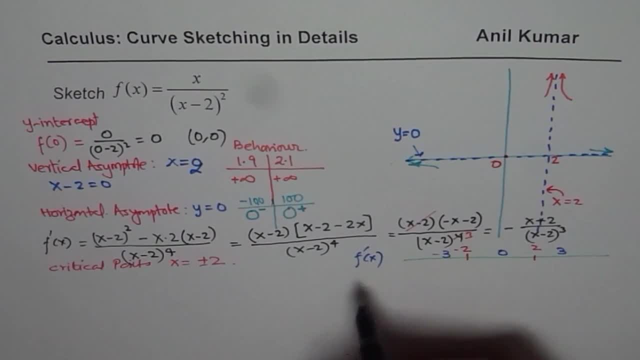 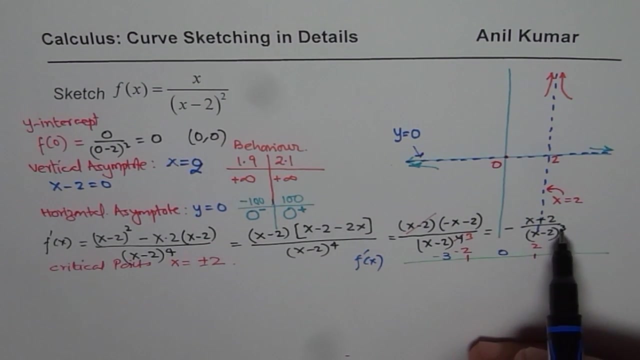 So if you analyze the derivative f, prime x, then what do you notice? If I substitute minus 3 here, then the numerator will be negative. As far as the denominator is concerned, that will also be negative. So we get 1,, 2 and 3 negatives resulting into negative when you multiply and divide, correct. 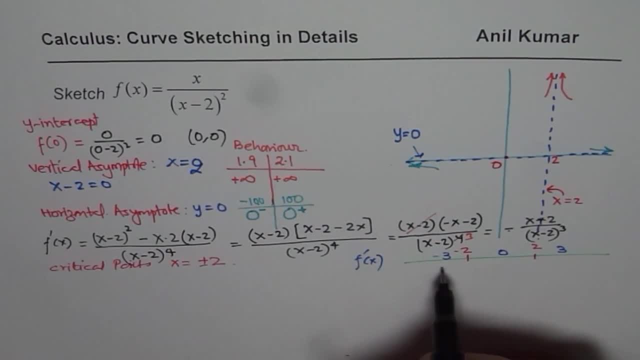 So that means at this point, since the derivative is negative, the function itself is kind of decreasing. Do you see that If I substitute 0 here, then in that case I will get negative divided by negative, which is positive. 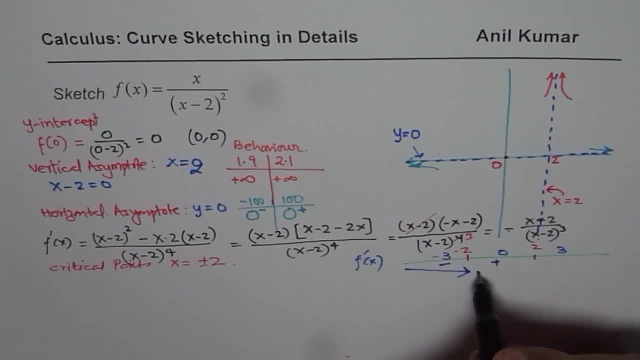 So at this point derivative is positive, So the function will be increasing, right. So we have a local minimum at minus 2,. right Now, if I substitute 3 here, numerator is going to be positive, denominator is also going to be positive- 3 minus 2, but this is negative, so the function will be decreasing, right? 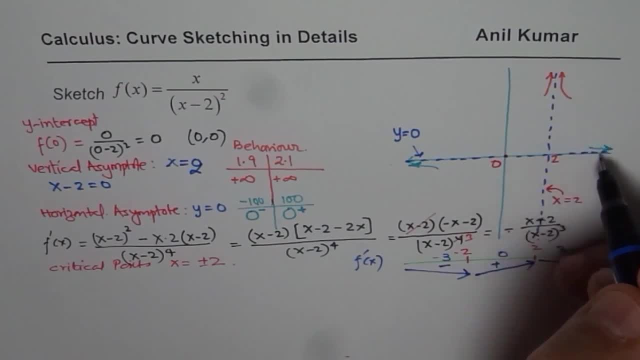 You can see if I am approaching from infinity to 0, the function is indeed decreasing, So it helps us to understand that part. However, there is no local maximum here, since we have a vertical asymptote, So don't get confused about it. 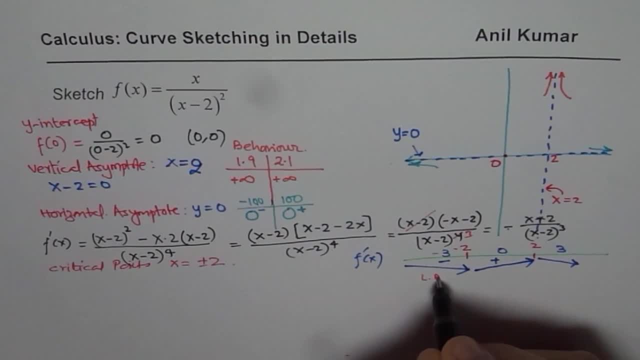 But we did find a local minimum, right. So we do have a local minimum, And that is At minus 2.. So what we can do here is we can find the value of the function at minus 2.. So if I substitute minus 2, what do I get right? 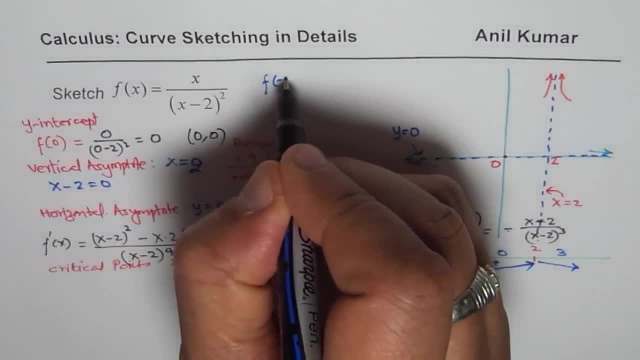 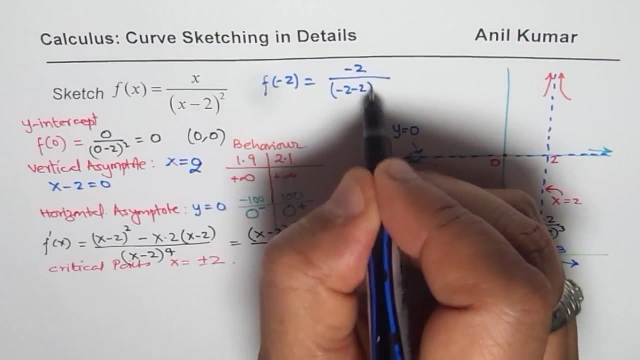 So let me write down f of minus 2 and calculate: So f of minus 2 is equals to minus 2 divided by. If I substitute minus 2 here, minus 2, minus 2 whole squared, which is minus 4 squared. 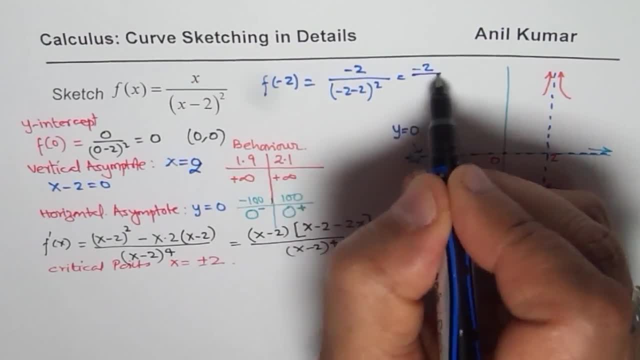 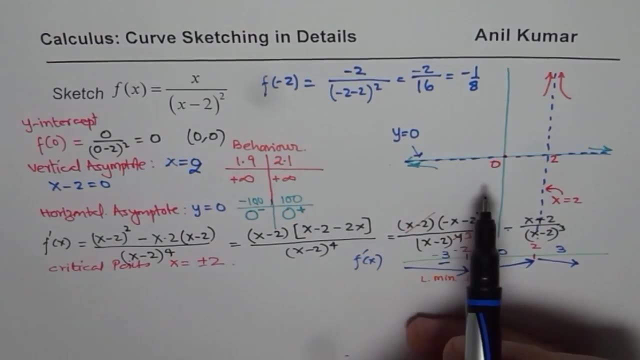 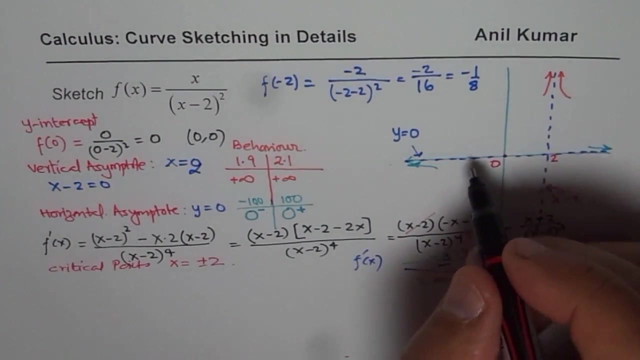 So I mean, so it becomes minus 2 over 6.. So that means we do have a local minimum at x equals to minus 2.. And the y value is minus 1 over 8, right? So kind of let us say, let us say, this is minus 2 for us. 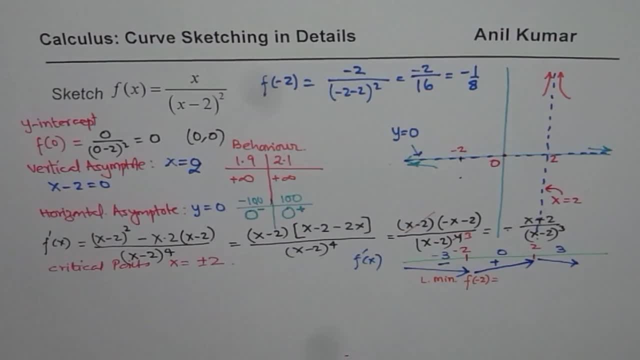 So the local minimum is somewhere there, right. So that is how we can find the local minimum for the given function. Now, to find concavity- change in concavity. we'll find the second function, We'll find the second derivative of this function. 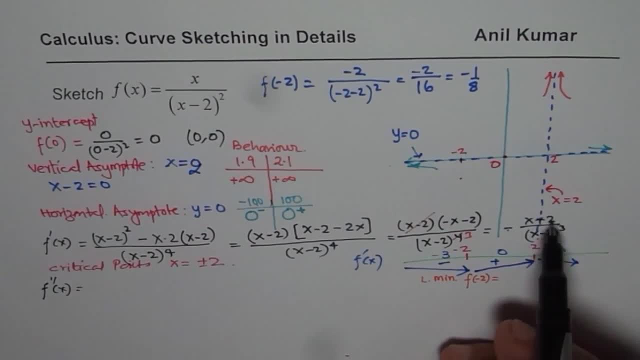 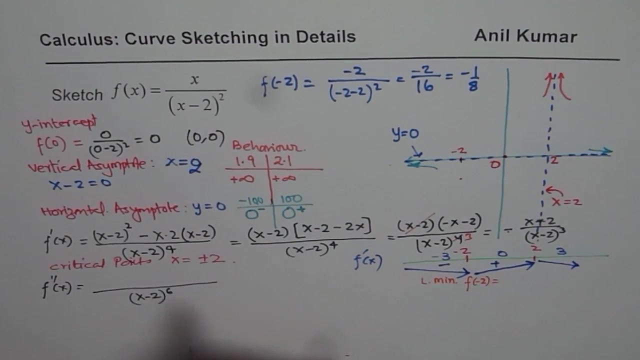 So the second derivative of the function is: we'll start from here. So the derivative is minus x plus 2 over x minus 2 whole cubed. Second derivative will be square of the denominator, which is x minus 2 to the power of 6.. 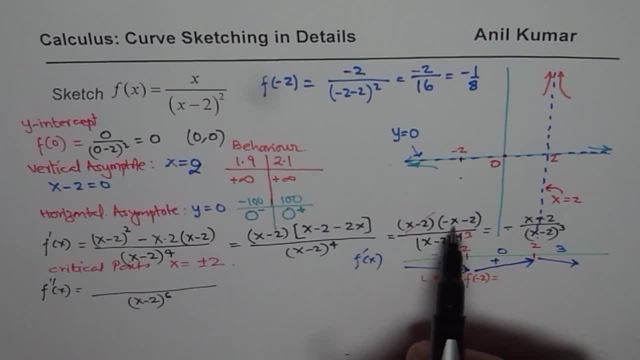 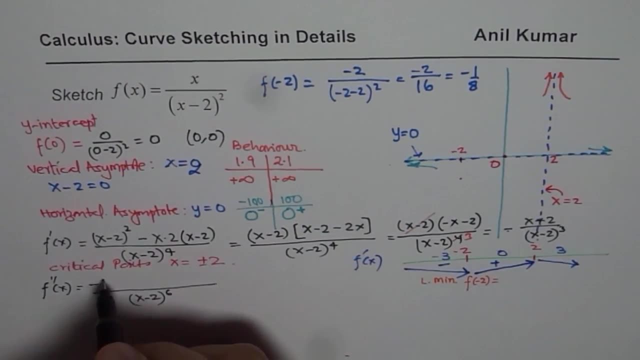 Now we can take we will use minus x minus 2.. It will be kind of simpler. So the derivative of minus x minus 2 is minus 1.. So that is negative times x minus 2, whole cubed minus the function itself. 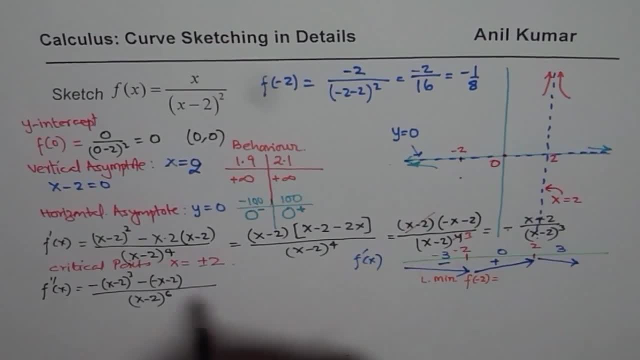 which is minus x minus 2 times derivative of denominator, which is 3 times x minus 2 whole squared times the derivative, which is 1.. So that is the second derivative, correct? Now we can actually simplify this also. 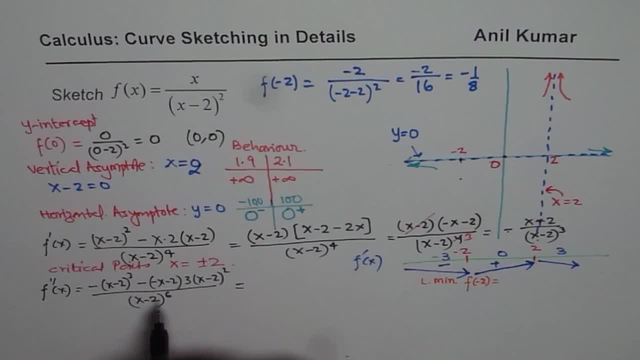 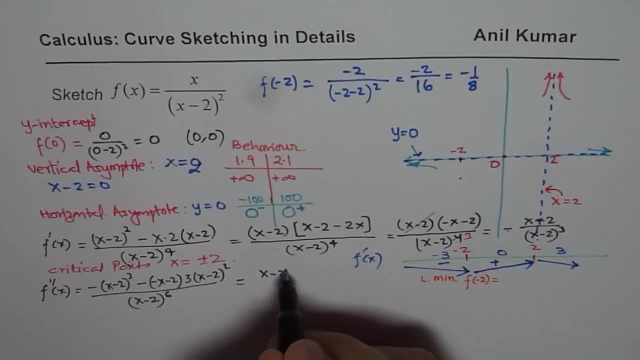 So let me simplify by taking x minus 2 whole squared. So we'll take x minus 2 whole squared common. We could also take negative common. Let's take negative also common. So in that case in the bracket I get x minus 2.. 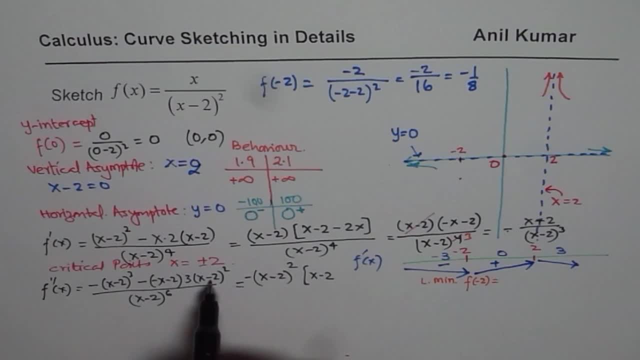 And here we took negative x minus 2 whole squared as common. So we are left with 3 times. So these are both now negative, right? So 3 times that means we can write this as minus. 3 times that means we can write this as minus. 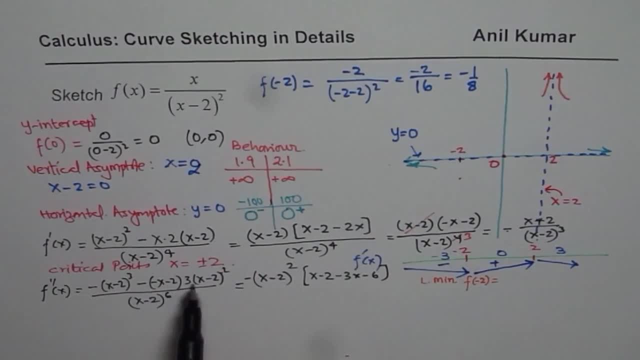 3 times. that means we can write this as minus 3x and minus 6, correct, So you could expand this and write: Divide it by x minus 2 to the power of 6.. Let's simplify this. 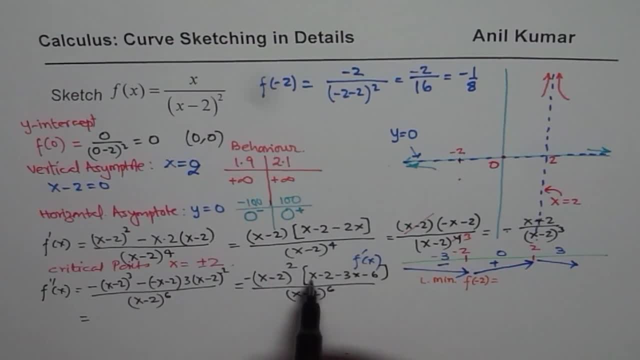 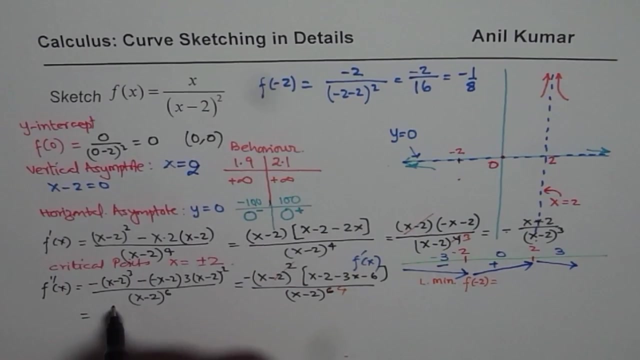 So that gives us here: x minus 3x is 2x, and minus 6 minus 2 is minus 8.. So what we have here is we could actually cancel this factor and get 4. here It becomes plus 2x and minus minus 8, plus 8, right. 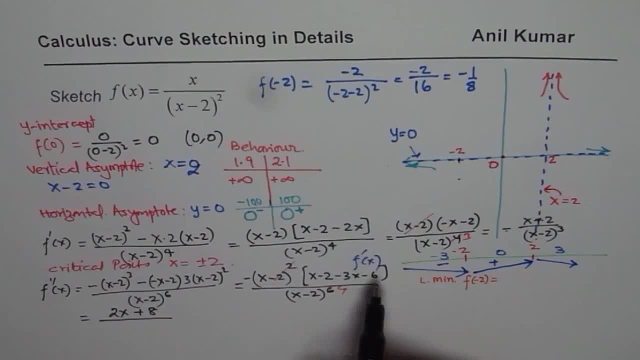 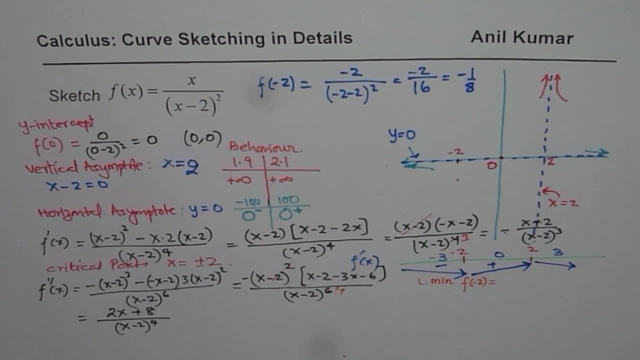 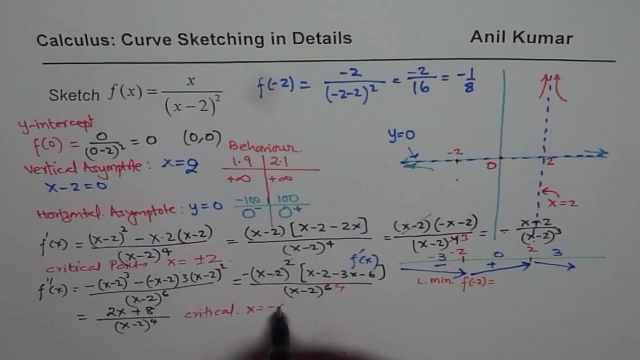 That divided by x minus 2 to the power of 4.. So that is what we get once you simplify Clearly here. the critical number for us is when numerator is 0 and when denominator is 0, right. So the critical number to analyze is at x equals to minus 4.. 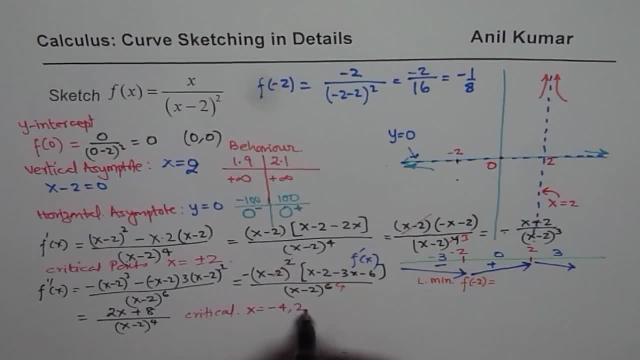 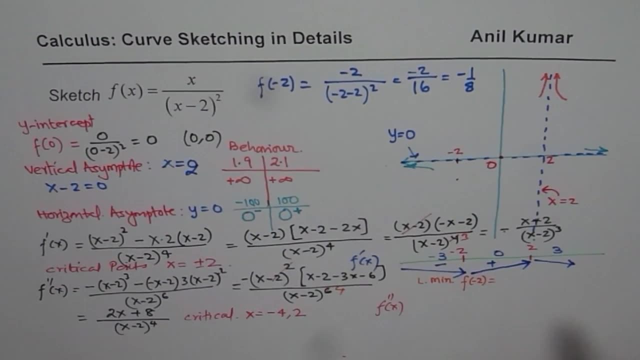 And at x equals to plus 2.. So now let us analyze the second derivative. So we will analyze the second derivative to find concavity right. So we will take the points. take the points minus 4.. Let's say this is now for us minus 4 and plus 2 is here. 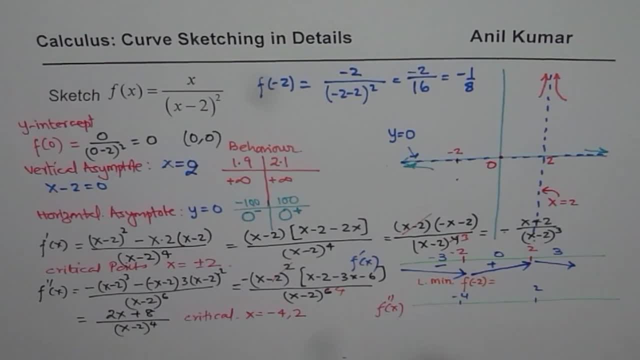 So the test points could be: let us say, minus 5,, 0 and 3.. If I substitute minus 5 here, we know denominator is positive to the power of 4, minus 5 will give us negative value, correct. 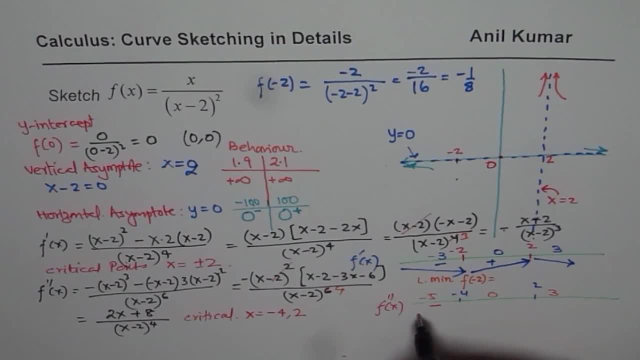 So at this portion it is negative. Negative means concave down. correct, Negative means concave down. If I substitute 0 here, I get plus 8.. Positive means concave up, So that is positive. If I substitute 3, again I get positive value over, which is concave up. 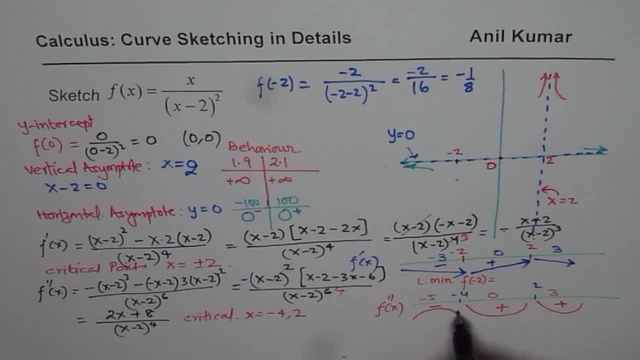 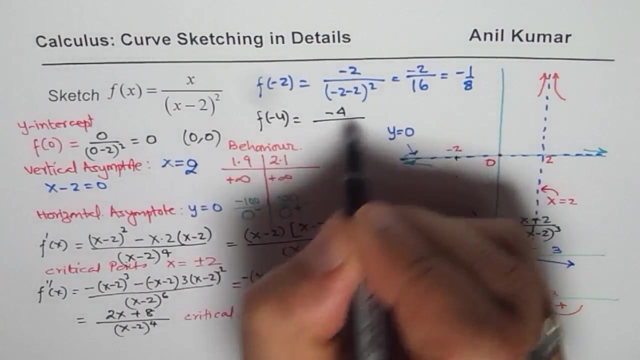 Now, since the concavity is changing at minus 4, we do have point of inflection at minus 4.. So let us find the value of the function at minus 4.. Substitute here: So f of minus 4 is equals to minus 4 divided by minus 4 minus 2, whole square right. 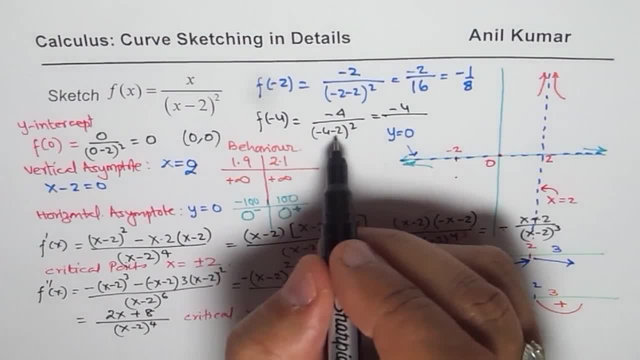 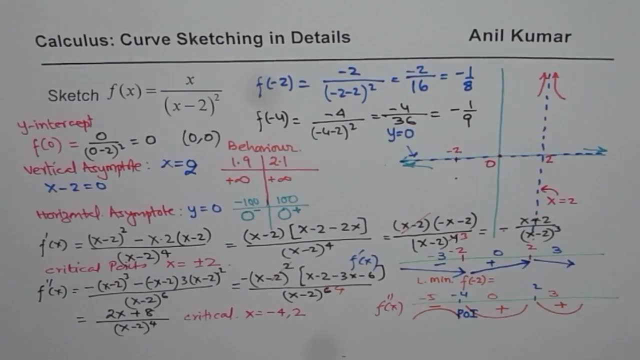 Which is minus 4 divided by 6 square is 36.. That is minus 1 over 9, right. So it is minus 1.. 1 over 9, correct. Slightly smaller than that, So kind of somewhere here, right. 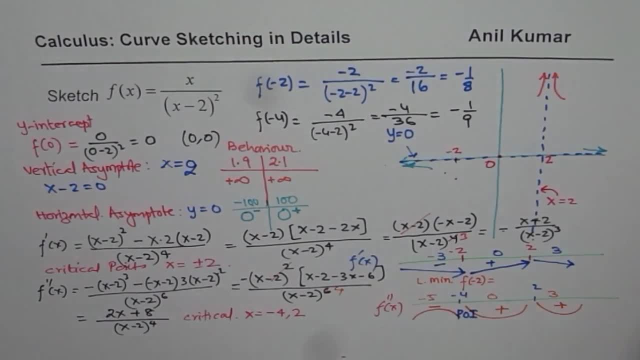 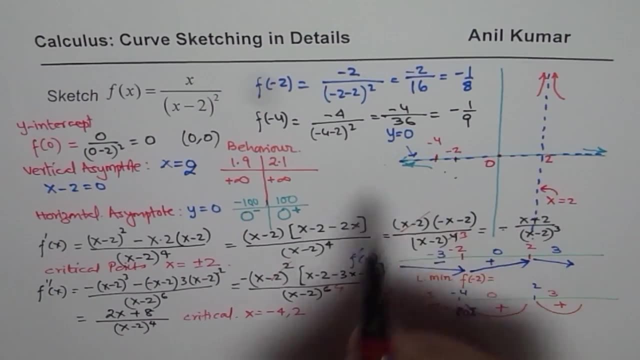 So at minus 4.. So now what we can do is: we know our point of inflection. Let us say: this is minus 4 for us at this point. So the concavity changes at this point right Now. with all this information, we can now sketch our graph. 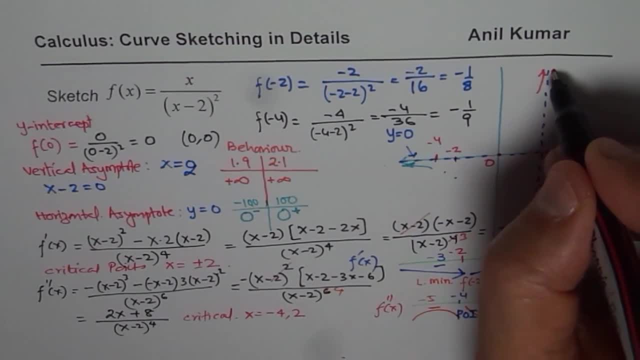 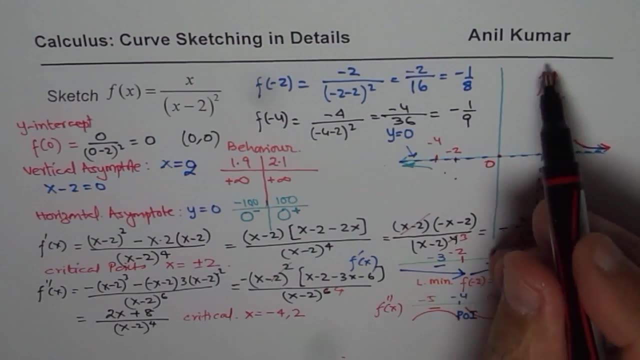 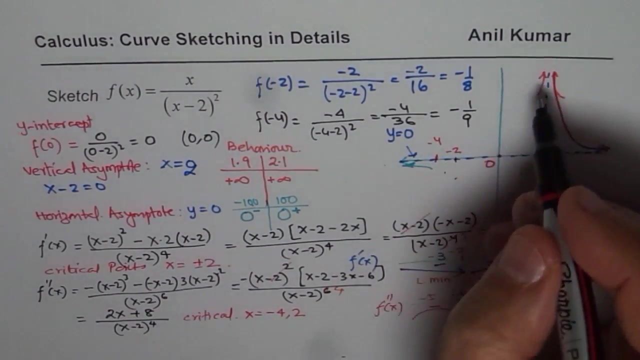 So the right side of 2 is kind of like this, correct. So we could just go like this and sketch concave up Function approaching positive infinity, for x equals to 2 plus and 0 from positive side. Here it has to go from the origin, right? 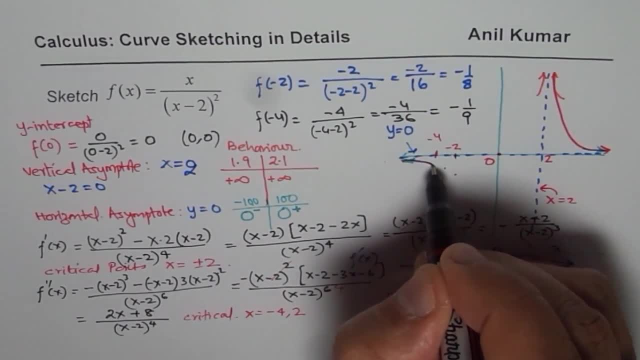 So and the concavity changes around at this point. So let me approximately sketch like this: So this is concave down for us, okay, We say, this is concave down, and then it is concave up, right, And kind of going up like this: 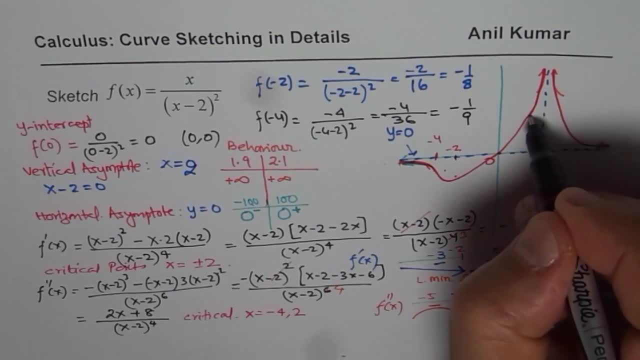 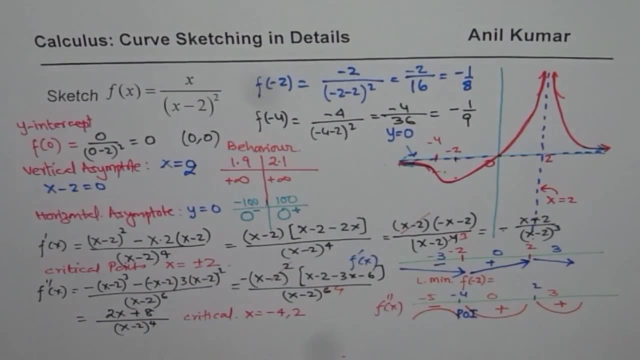 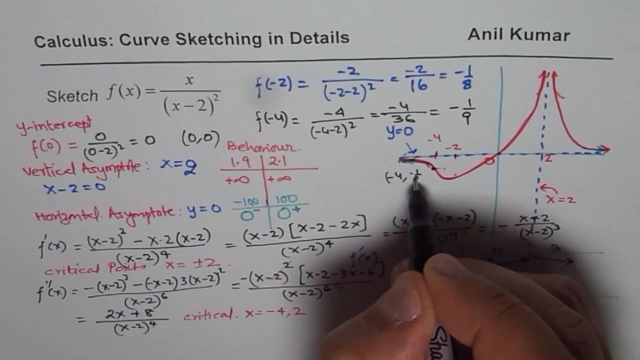 Do you see that? So that is how the graph is going to be. So it should be kind of like this: Local minimum at minus 2, concavity changing at that point. So I will write this point as point of inflection, which will be at minus 4 minus 1.9.. 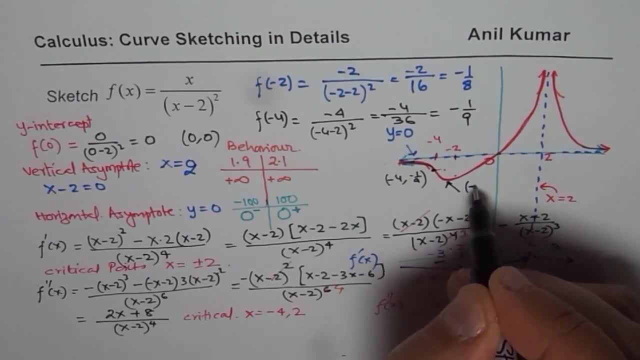 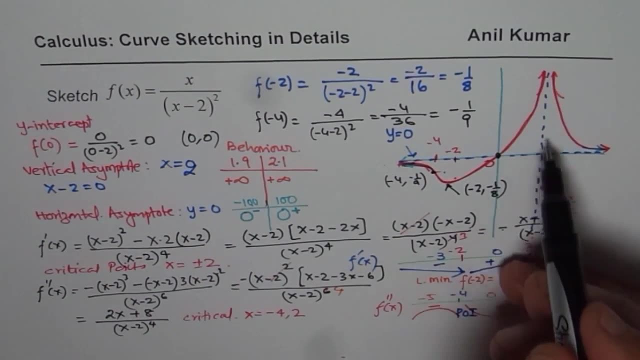 And that is the minimum for us, at minus 2, minus 1, over 8, right. And that is the x and y intercepts, And this is our vertical asymptote, And then that is our horizontal asymptote: y equals 2.. 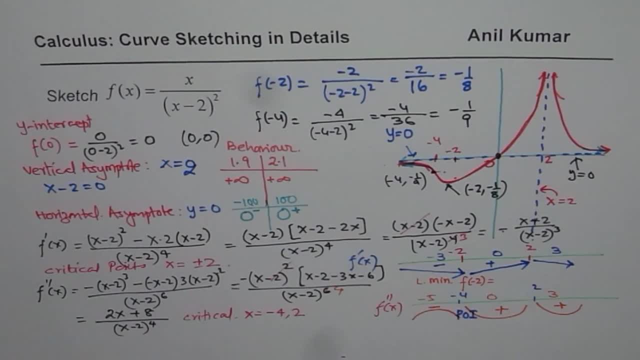 And that is our vertical asymptote 0.. I hope with this you understand how to sketch graph of a function. So look at the equation itself. It gives you an idea right how to go about Now. finding x and y intercepts is first thing. 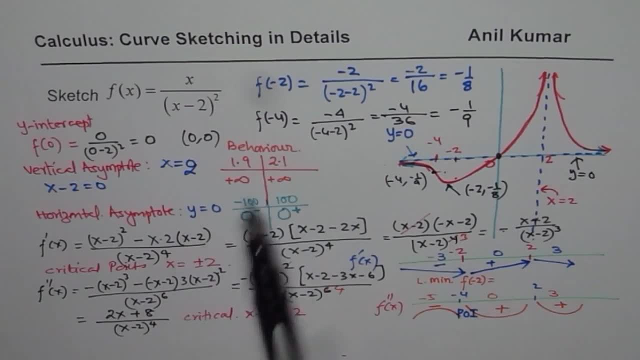 Then you can find asymptotes, behavior near the asymptotes, local maximum and minimum points, concavity and thereby point of inflection. Once you have these things in place you can sketch a neat curve to represent the graph of the given equation. 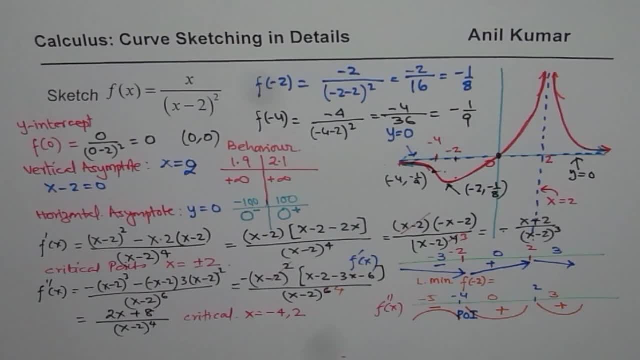 I hope that helps. Thank you and all the best. 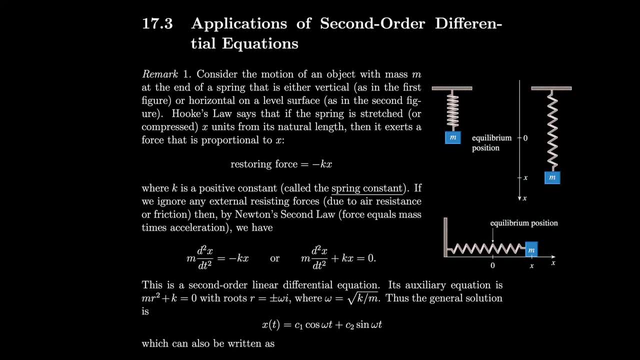 Section 17.3.. Applications of second-order differential equations. Consider the motion of an object with mass m at the end of a spring that is either vertical, as in the first figure, or horizontal on the level's surface, as in the second figure. Then Hooke's law says that if the